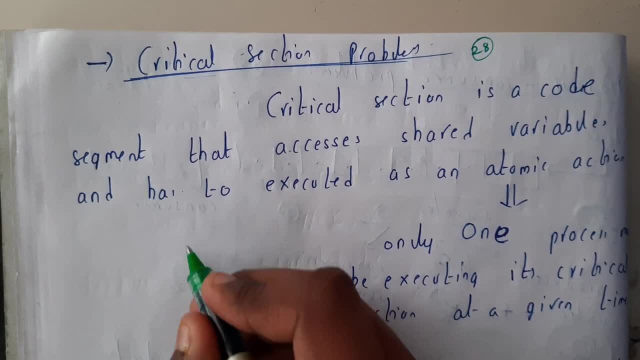 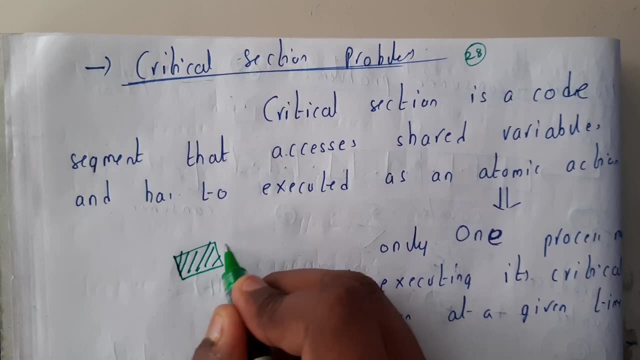 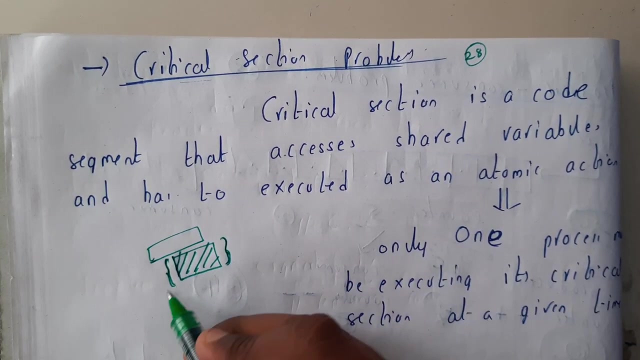 is what is critical section. So the critical section is nothing, but it is a small block of code. Okay, so you will be writing a small block of code that we will be calling it as a critical section, which has a particular entry and exit guys, So only one process can. 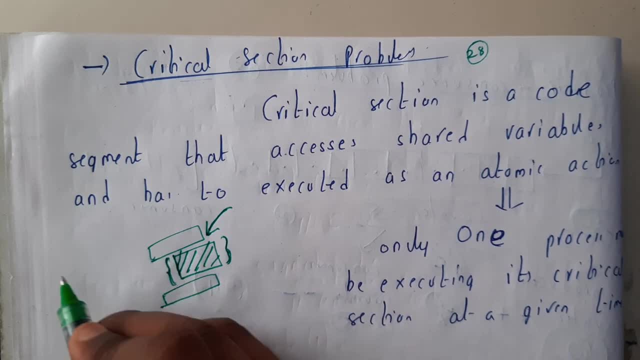 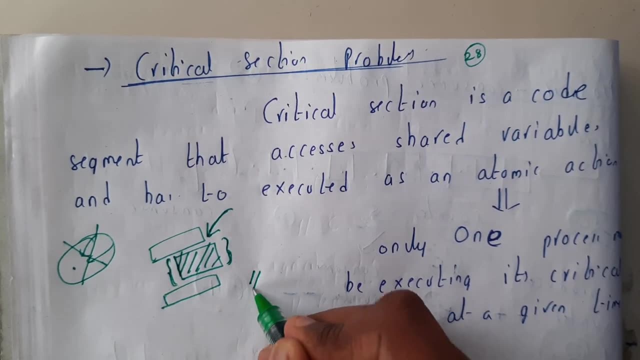 enter this section at a moment. So previously we discussed that at a moment there are multiple processes trying to access the same variable. To remove this, we will be using this critical section. So the entry will allow only one process to enter inside and the exit will. 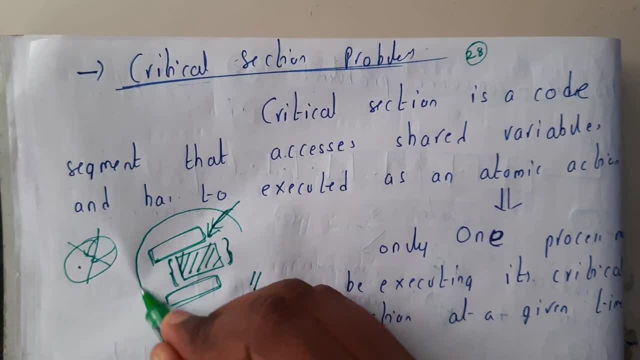 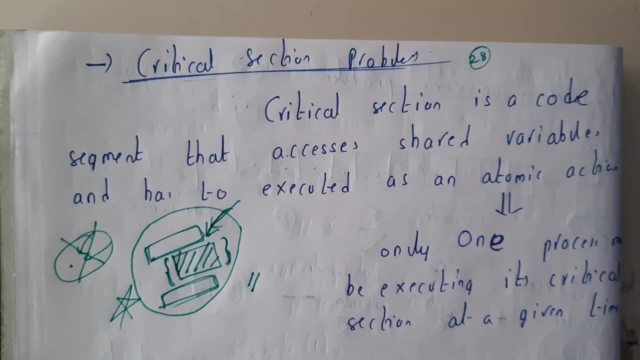 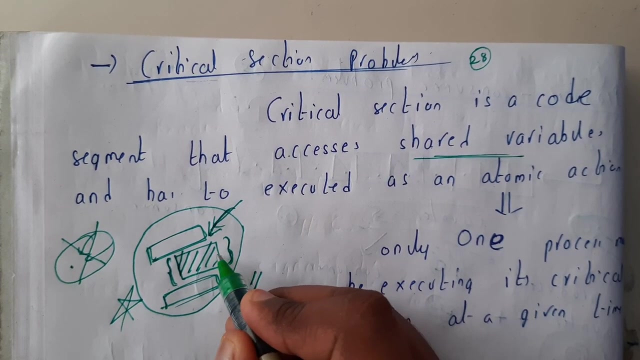 let it exit and then the next process enters. So this is one of the most important solutions for the previous problem and this is an important concept in process synchronization. So critical section is a code segment that accesses shared variables. Yeah, in this we should use shared 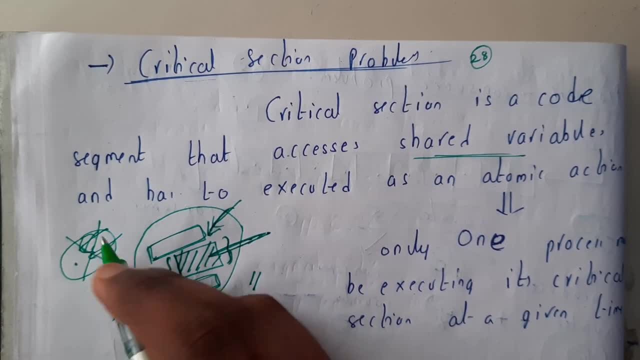 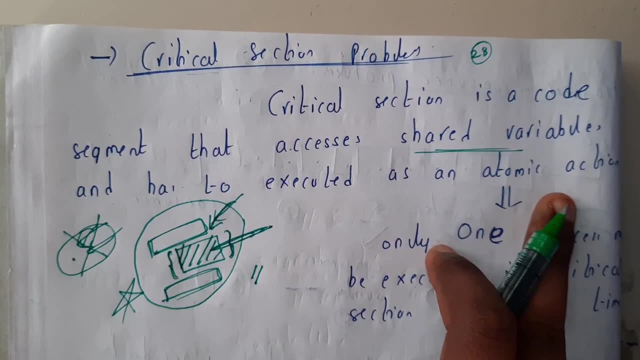 variables: right, So the variables which are trying to be accepted by different processes will be used here. So variables. and has to execute as an atomic action. So they will be executed in a single way. Atomic means only one, Yeah, single process at a time by. 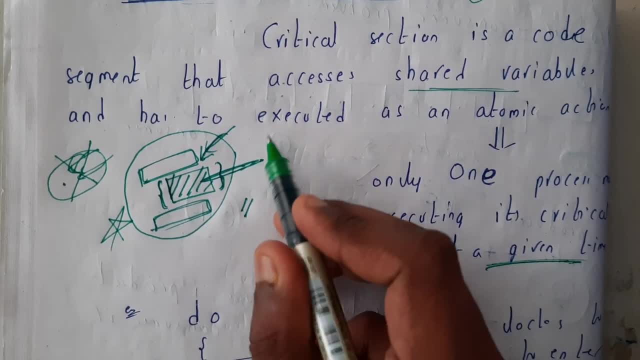 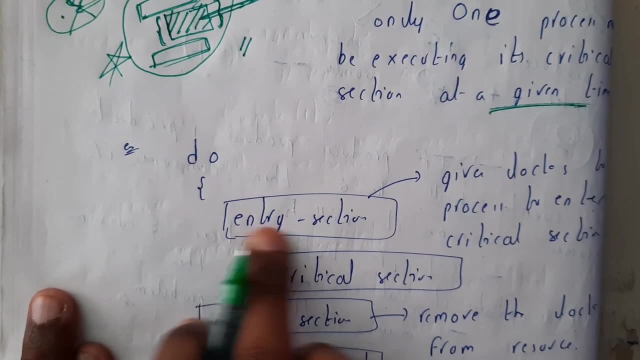 executing its critical section at a given moment of time, So at one second at one moment of time. only one process will be updating the values, So the syntax of it will be in this way: Do entry section the critical section. exit section. remaining code, If there is. 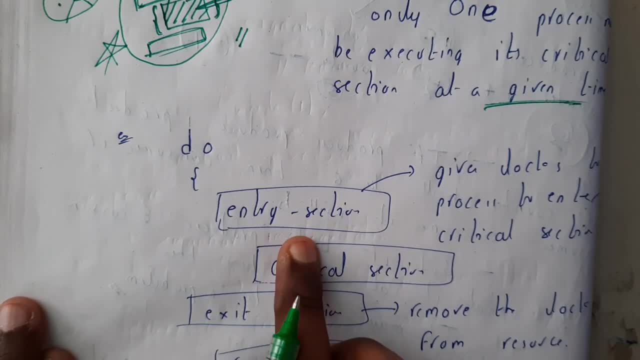 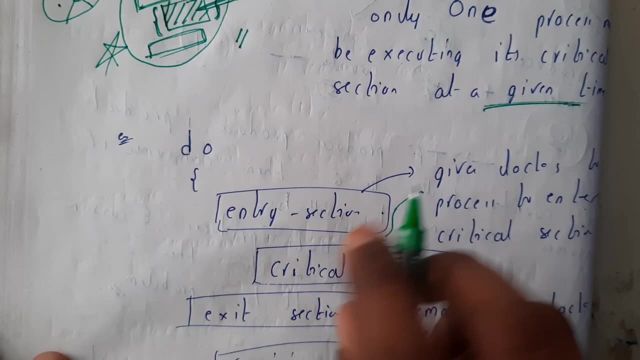 any remaining code. that and we'll be doing an infinite loop while So. this entry section gives lock to the process to enter the critical section. So once a process enters the critical section, it applies the lock and exit will remove that lock so that the next process. 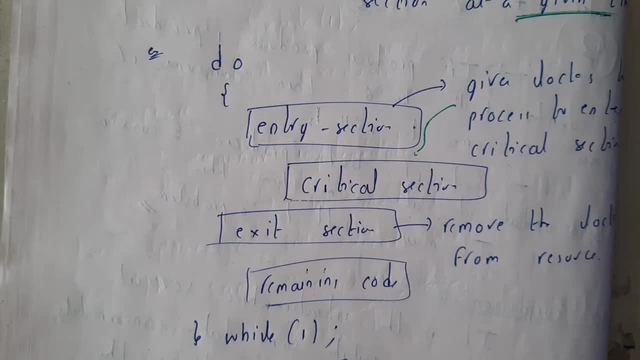 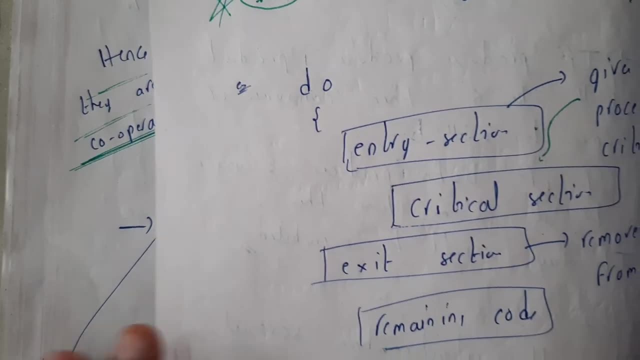 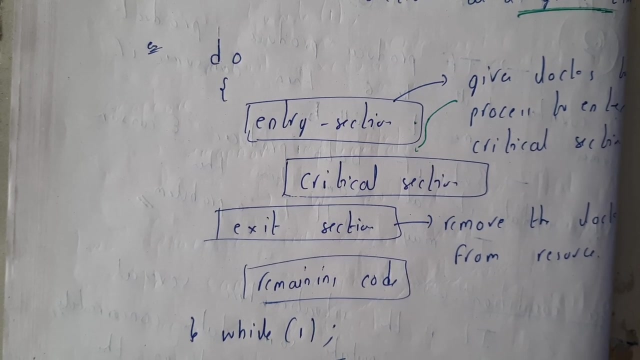 can come. So this is a lock, a small lock mechanism. Okay, so I hope everyone got a small idea. So in the next tutorial we'll be going through some solutions for this critical section, how we can use this critical section in our view, in our use. So let us meet in the next. 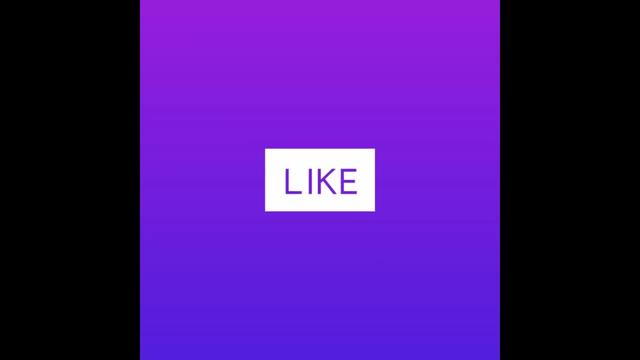 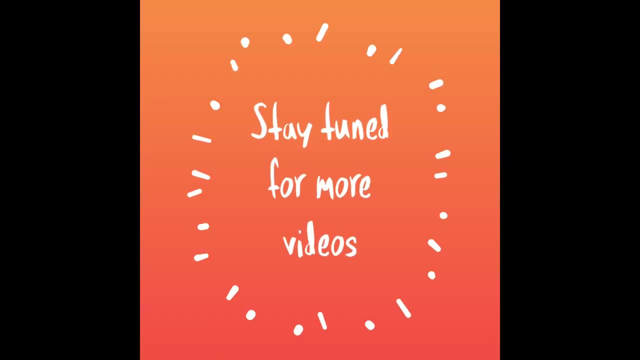 tutorial. Thank you. Thanks for watching, Thank you.